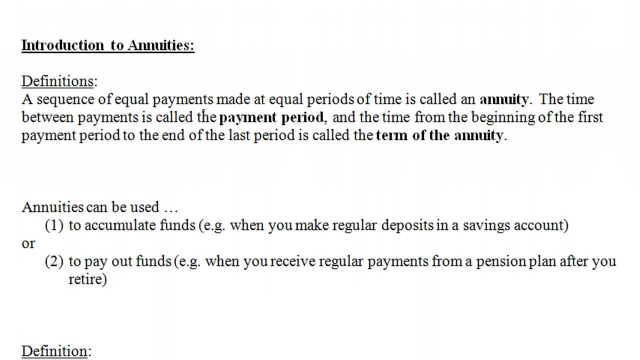 at equal periods of time is called an annuity. Okay, now these have to be equal payments. Okay, if you're putting in $150 one month and $225 another month, then that's not an annuity, Okay. and it also has to be equal periods of time, So you can't put it in once, then three weeks later again, then two weeks later, then five weeks later. It has to be equal periods of time. Let's say, for example, at the end of every month. Okay, now, the time between payments is called the payment period. So that would be one. 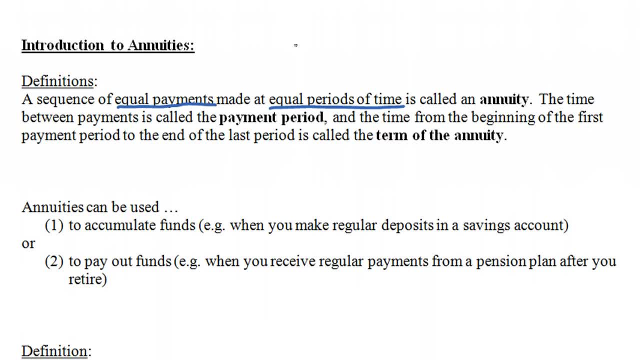 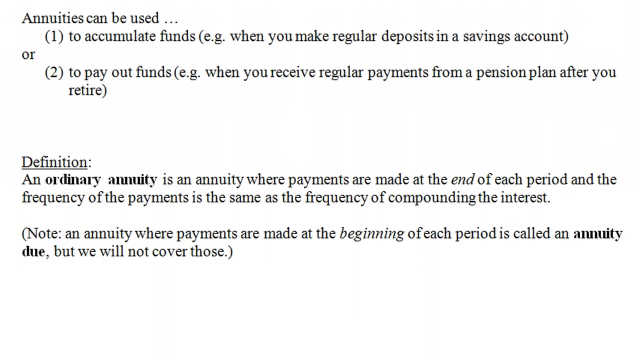 month in that scenario, And the time from the beginning of the first payment period to the end of the last payment period is the term of the annuity. Maybe, if you're trying to, you know, you know you're going to retire 30 years from now and you start putting in these payments for 30 years, the term of that annuity would be 30 years. Okay, now, annuities can be used a couple different ways. One way is to accumulate funds, So that's just like what we've been talking about when you're making regular deposits into some savings account or some retirement account. Okay, another way. 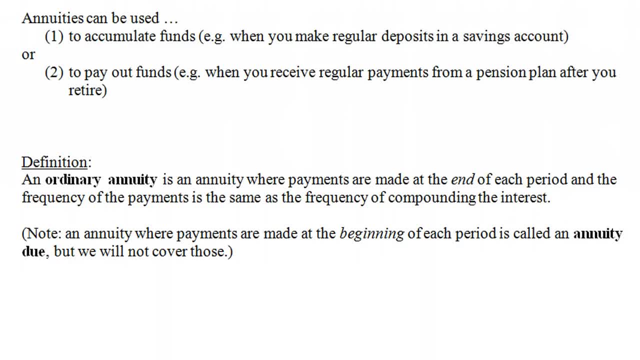 annuities could be used is kind of just the opposite, though, is to pay out funds, For example, once you already are retired, okay, and you receive, let's say, regular payments from a pension fund or pension plan, that could also be considered an annuity. So maybe every month you receive $1,500 or so, let's say, Okay, that would be called. that would also be called an annuity. Now, in this video, we're primarily going to be interested in this type of annuity, the first kind, Okay, so what is an ordinary annuity? 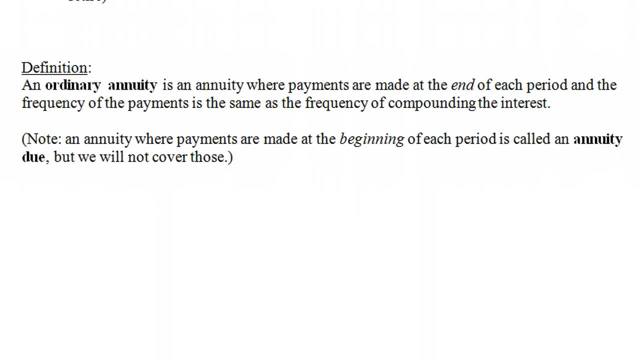 An ordinary annuity is an annuity where payments are made at the end of each period. Okay, so, for example, the end of each month instead of the middle of each month, or the beginning of each month, Okay, and the frequency of payments is the same as the frequency of the compounding of the interest. So, in other words, if you make payments every month, then the interest is supposed to compound monthly. Okay, if it compounds daily but you're making monthly payments, you don't have an ordinary annuity. 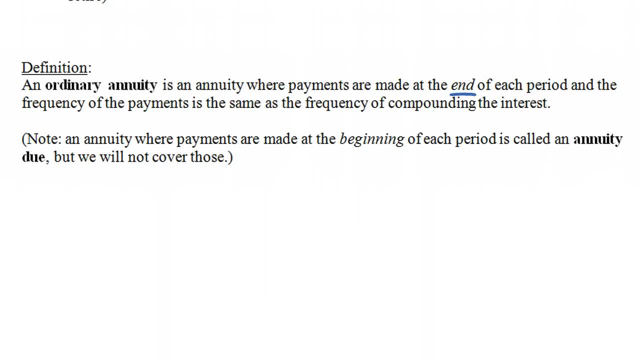 It's called ordinaries because these are very common types of annuities, because they're easy to calculate. Okay, if you have, the frequency of payments is the same as the frequency of the compounding of the interest. Okay, also a special note here: an annuity where payments are made at the beginning of each period, okay, maybe the beginning of a month, every month, or the beginning of every year, that would be called an annuity due. So when you see this word D-U-E, that's what that means. But we're not going to cover those, We're not going to talk about those. Okay, so let's do an actual example. 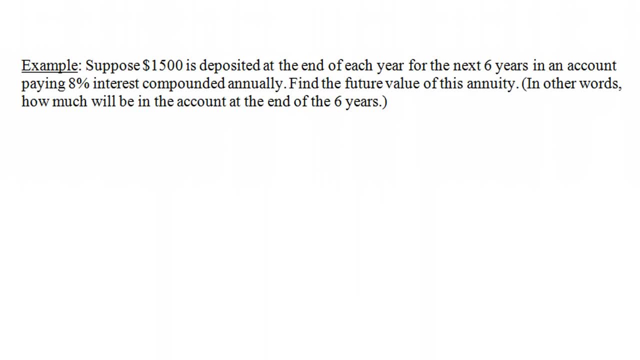 It says: suppose $1,500 is deposited at the end of each year. Okay, so we're making yearly payments, not monthly ones. Suppose $1,500 is deposited at the end of each year for the next six years in an account paying 8% interest, compounded annually. Okay, find the future value of this annuity, In other words, how much money will be in the account at the end of the six years? Okay, now, first of all, notice: this is an ordinary annuity. Okay, it's an annuity because we're putting in the same amount every month, right, $1,500. 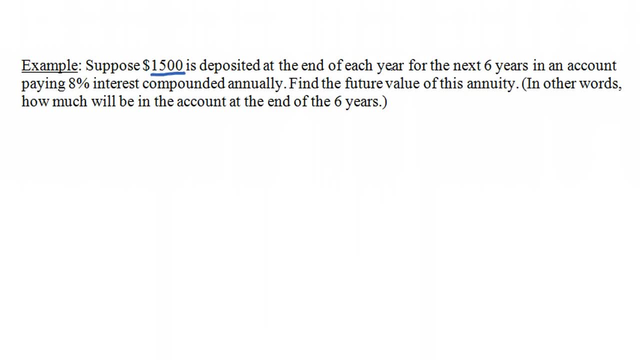 So every month, I'm sorry, every year. this is happening every year and our interest is compounding annually. Okay, also, we are paying at the end of each year. Okay, so what we have is an ordinary annuity. Okay, now, how much is this annuity going to be worth? Well, let's kind of draw like a timeline here. Okay, let's say this represents six years: Two, three, four, five, six, because it's not very straight. 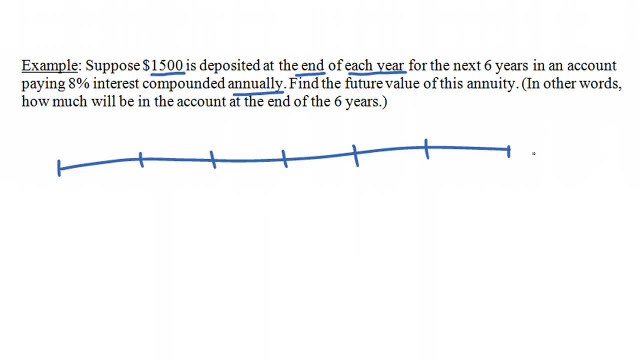 Okay, let's suppose this represents the beginning of the six years and this represents the end of the six years. So here's the first year, the second year, the third year, fourth, fifth, sixth, Okay, and notice, when will your first payment be? Well, notice, it's not right here. If that first payment right at the beginning, that would be an annuity due, Okay, but you're putting in $1,500 at the end of the first year, Okay, and you're doing that a total of six times Okay, at the end of each year. 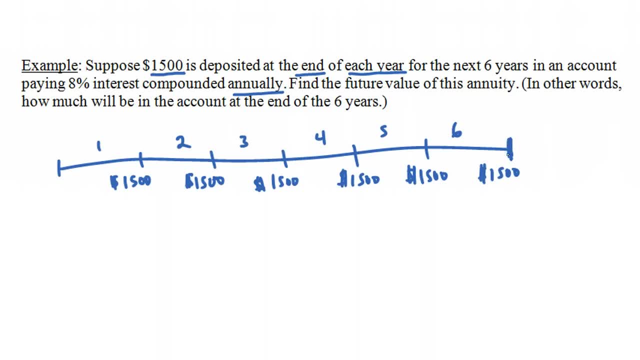 six years And the question is: how much money do you have? right here, at the very end, Well notice, if you weren't getting any interest, how much money would you have? Well, you made six payments of $1,500, and six times 1,500 is $9,000.. So I would expect to have $9,000 if I didn't make. 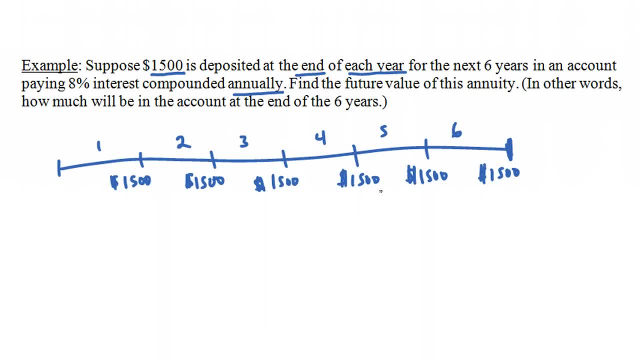 any interest. So the fact that I'm making interest means I know I should have more than $9,000 at the end of the six years. Now how do we figure this out? How do we figure out how much money we have? 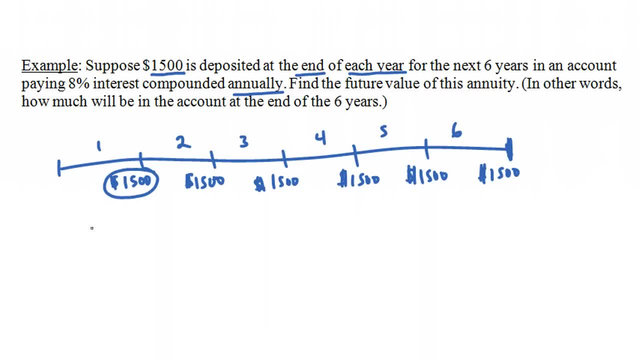 Well, let's look first of all at this first $1,500 payment. How much will that be worth at the end of this time? And then we'll look at the next $1,500 that we put in. How much will that be? 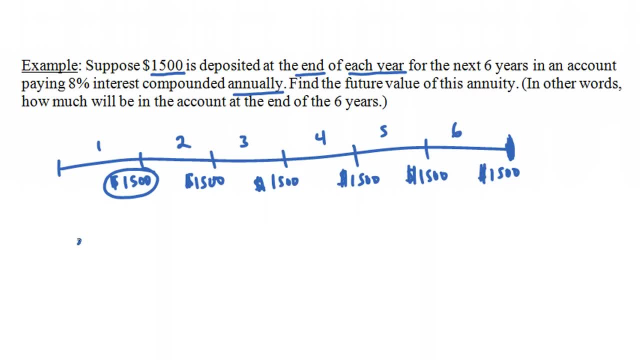 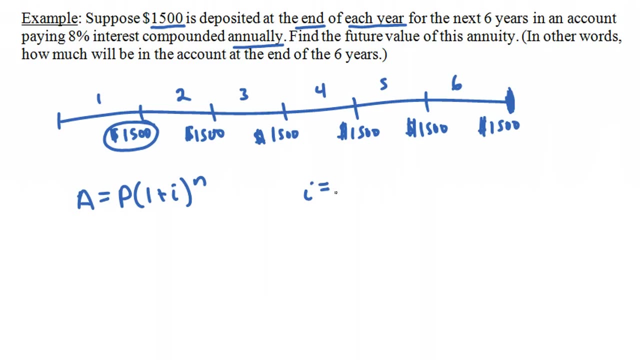 worth. And we can add all these up, So let's the first $1,500,. now remember, our formula for compound interest was: A equals P times 1 plus I to the N. Okay, And we're getting compound interest. Notice, we're compounding annually. Okay, 8%. So our I is actually 0.001%. 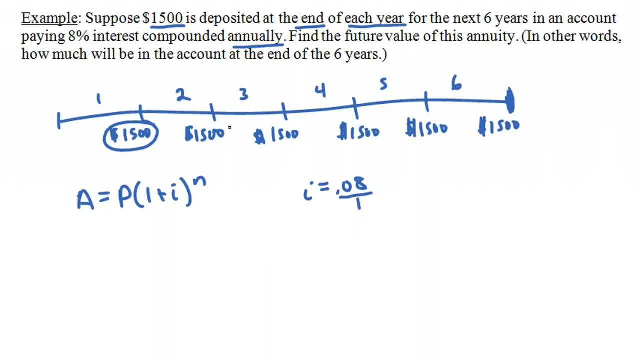 0.08, now you might think 0.08 over 1. if we were compounding monthly, this would be 0.08 over 12, but I is 0.08 over 1, so that's just 0.08.. 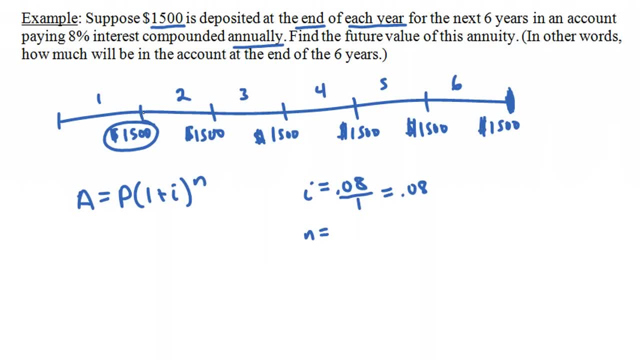 What is the N? Well, for this particular $1,500, the N is going to be 5 because it's going to accumulate for 5 years. Well, it's going to accumulate through 5 compounding periods because it's compounding once a year. 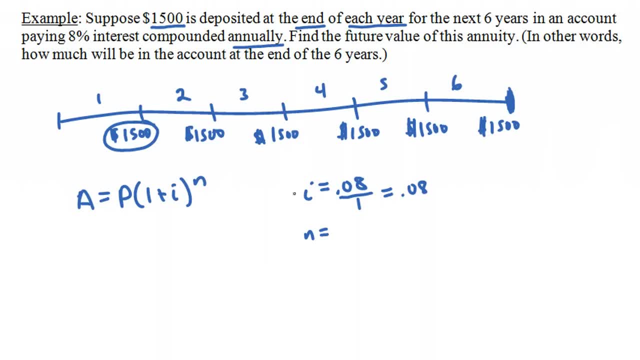 and for the next 5 years. Now, why not 6?? Well, because we didn't start here. we started here, Okay, so N is going to be 5.. In the P, of course, it will be 1,500. 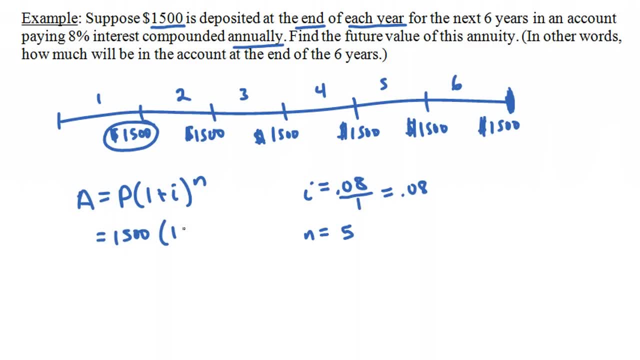 This 1,500, we plug it in, we get 1 plus 0.08 raised to the 5th power. or in other words, it's 1,500 times 1.08 to the 5th power. 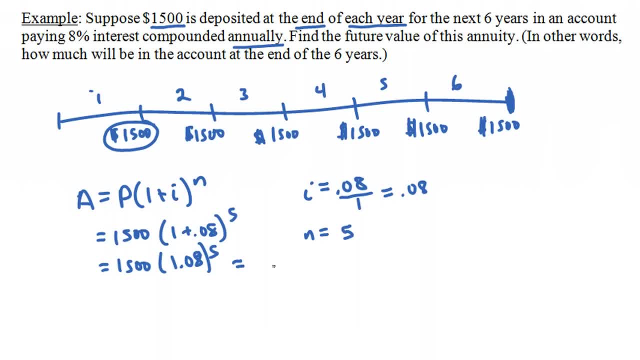 Whatever that ends up being, let me check what it is. Okay, I worked it out and I got $2,203.99.. In other words, this $2,203.99.. $1,500, it grew over time, right. 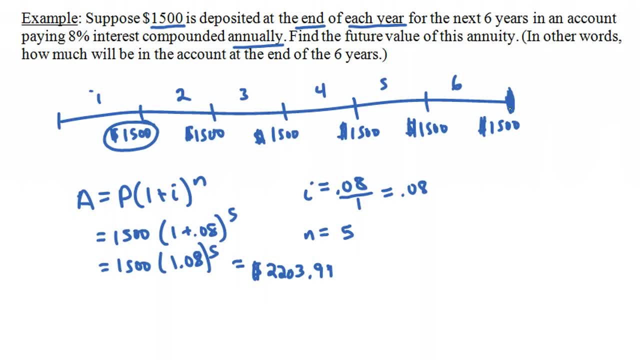 It grew to be $2,200, over $2,200 at the end of the year. Okay, basically it gained a little over $700 in interest and each of these $1,500 is going to grow over time. Now this $1,500 isn't going to grow to be quite as much as that first $1,500, because 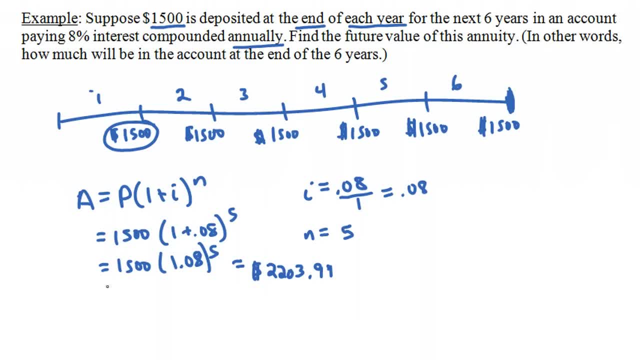 it doesn't have as long to grow, But anyways, that's what we get. But actually, instead of looking at this number, this $2,200 number, I want to look at just the formula for it here And I want to figure out how much money would we have total? 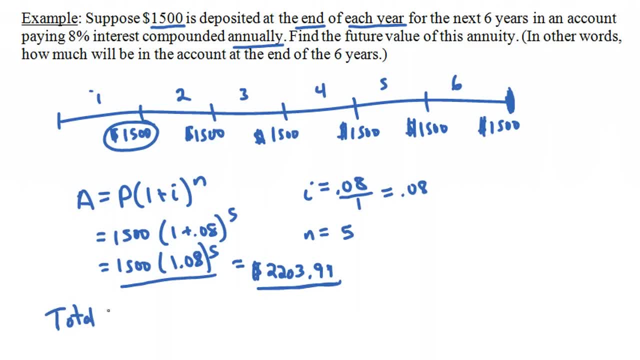 Okay, so I want to figure out how much money would we have total. Okay, so I want to figure out how much money would we have total. Okay, so I want to figure out how much money would we have total. Okay, total, the total amount we'd have at the end of the six years. first of all, it 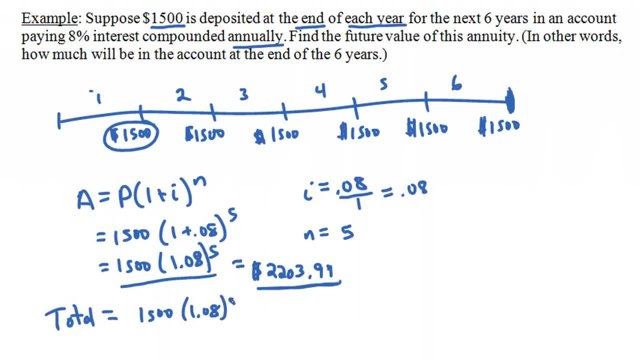 would be this: $1,500 times 1.08 to the fifth power. That would be how much this $1,500 grows to Now. the next one- this $1,500, you can see- would be $1,500 times 1.08 to the fourth power. 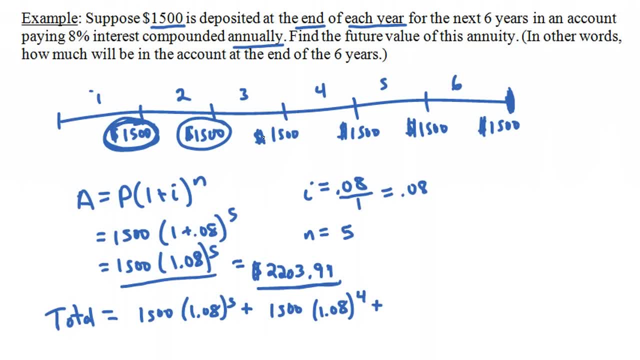 Okay, you could work this same calculation again. that's what you get, And the next one would be $1,500 times 1.08 to the fifth power, 1.08 to the third, and then 1,500 times 1.08 squared, plus 1,500 times 1.08 to the first. 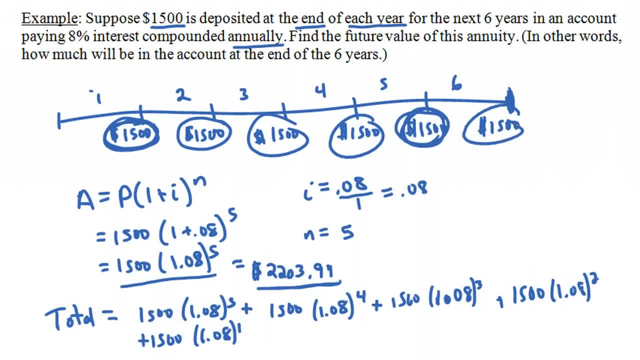 power. that would be this amount right here. And the last amount is really just. I mean, it's not going to grow at all. It's like 1,500 times 1.08 to the zero, but 1.08 to the zero is just 1, so we could just. 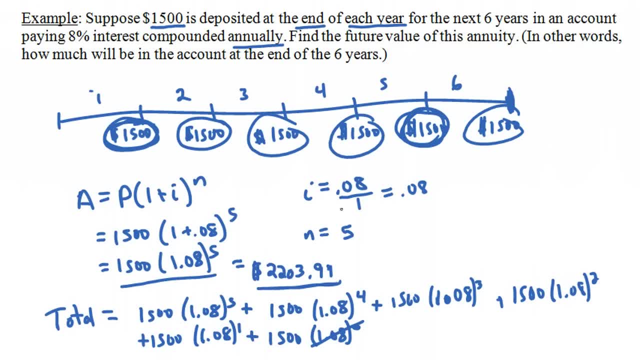 write plus 1,500.. 1.8 to the zero plus 1,500 golden coins. Okay that 1,500. I didn't have to change 1,500 with 2着 1.08.. 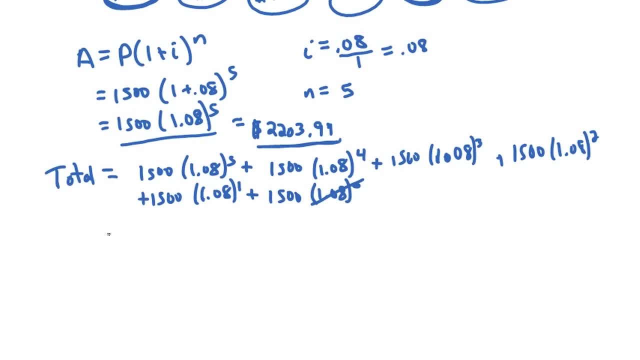 Okay, 1.08 times 1.08 to the three, any time to grow. okay. now notice what happens when we add all these things up. what do all these terms have in common? well, they all have a 1500 in common. okay, so let's factor out the 1500. now notice, let's. 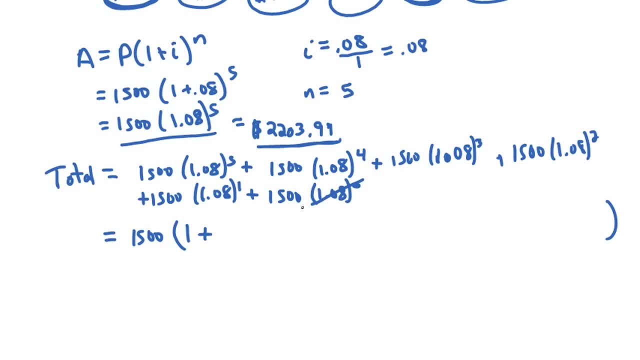 actually kind of do this in reverse here: 1500 times 1, that would be this term. 1500 times 1.08 to the 1, that would be this term. okay, and then we have 1.08 squared right times this 1500, remember. 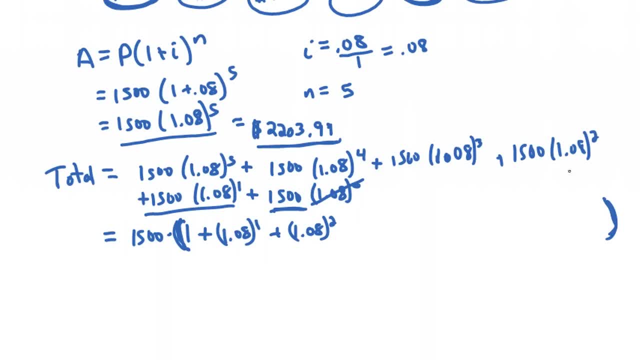 this 1500 is distributing here. okay, that would give us this term, okay, and so on. so we're gonna have plus 1.08 cubed, plus 1.08 to the fourth and finally, plus 1.08 to the fifth power. okay, well, if 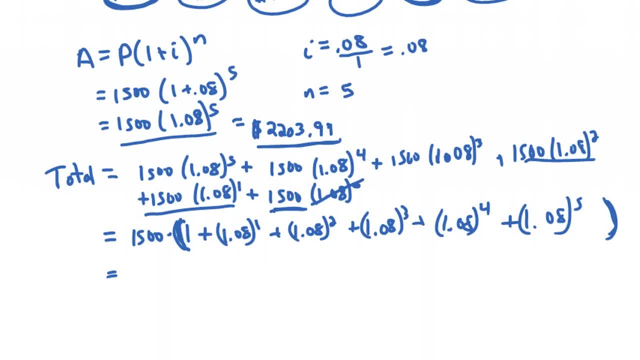 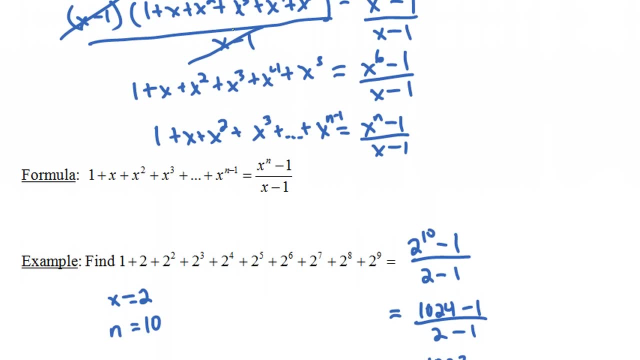 you remember the formula that we had from the previous video? we had this, this formula. we can find it here. remember this, this formula, right here. let me circle it: 1 plus x plus x squared plus x cubed, all the way up to x to the n. minus 1 equals x to the n. 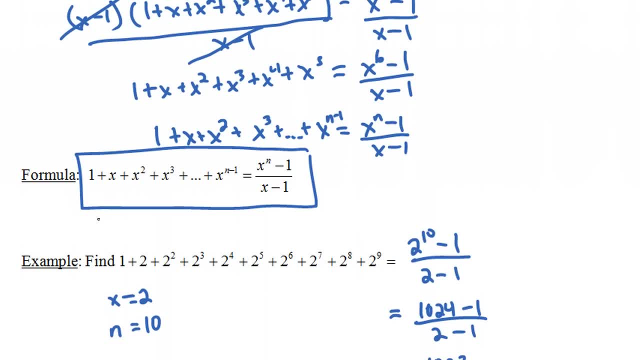 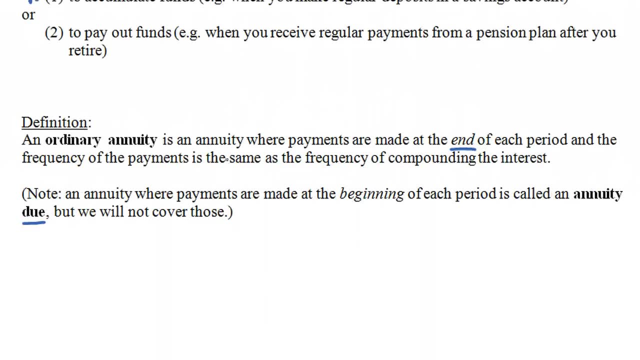 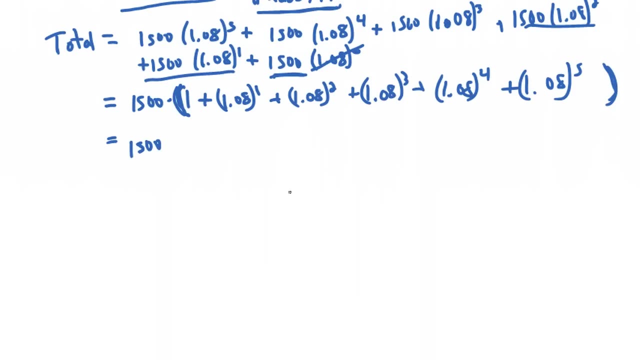 minus 1 over x minus 1.. now, this x is really just 1.08 now in our video, okay, and let's figure out what the n would be as well, okay, so, so let's write this out: this is really uh, 1500, uh, and remember. 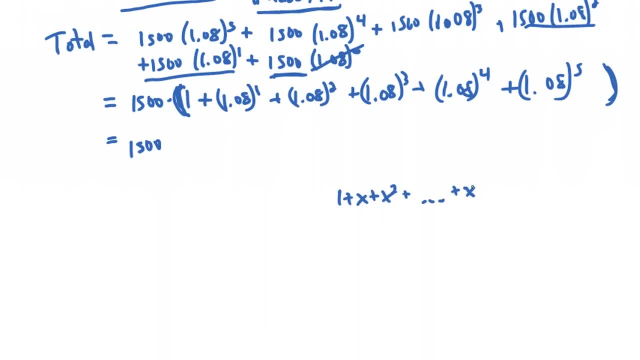 so let me write the formula again: one plus x plus x, squared all the way up to x to the n minus one, equal x to the n minus 1 over x minus 1.. so notice, our n actually would be 6.. you might think: well, i thought. 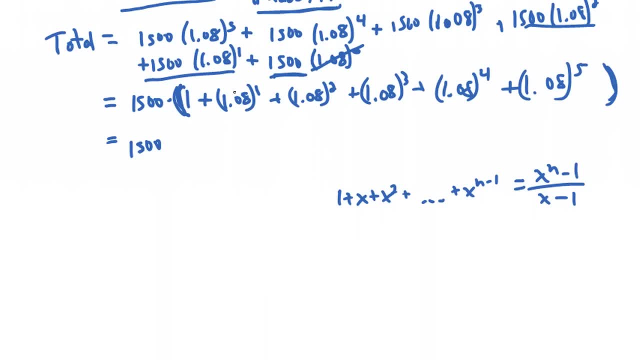 n was 5 here. right, well, that's the n minus 1.. okay, what's inside the parentheses here? that's going to correspond to this. okay, this part here is going to correspond to this, where the x is 1.08, okay, and the n minus 1 is 5, so n is actually 6.. so, so what we can say is: this is equal to this. right, these two. 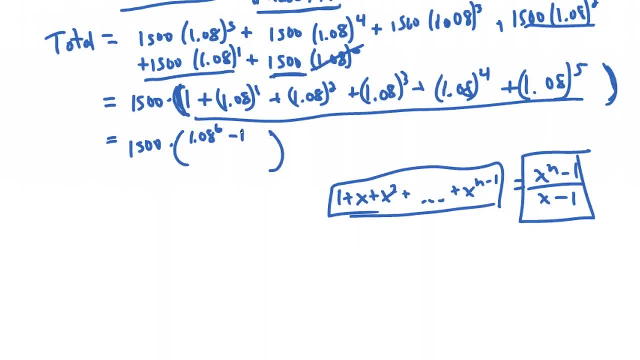 are the same, so i'm going to put 1.08 to the 6th minus 1 over 1.08 minus 1.. okay, so i used this formula that we had- we had worked out in the previous video- to say that this expression. 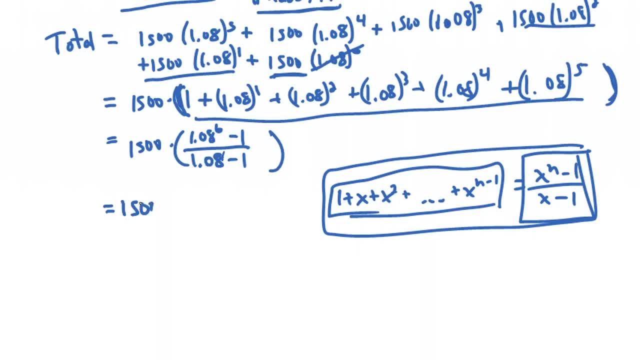 is equal to this expression. now, another way to write this would be 1500 times 1.08 to the sixth power. i guess i could put that in parentheses, minus 1.. now what is in the denominator? 1.08 minus 1? that's just 0.08. 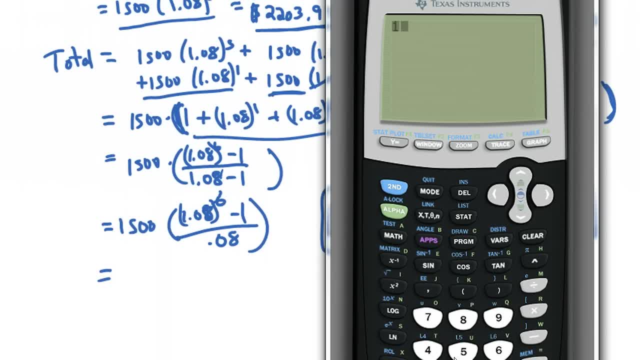 okay, now we could figure this out. let me do this. okay. so let's type this into a calculator. we have 1500. now we have to be a little bit careful about our parentheses here. but times, so in parenthesis, so in in the in the numerator. so i might need to put another uh parenthesis. here i'm going to put 1.08. 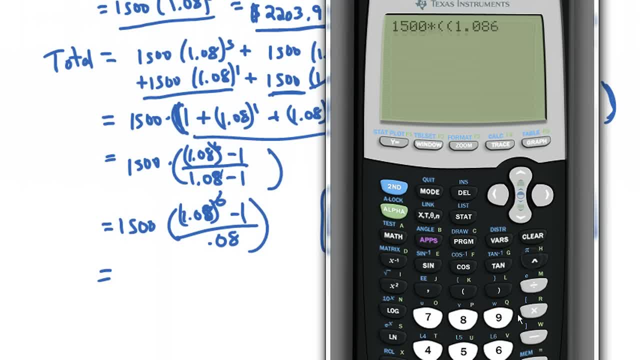 raised to the sixth, whoops raised to the sixth, okay, minus one, okay, and the parenthesis then divide it by okay, and then we'll put uh, 0.08 and end this parenthesis okay, and what do we get? eleven thousand, a little over eleven thousand dollars. notice, if we didn't get any interest, we said we'd have nine. 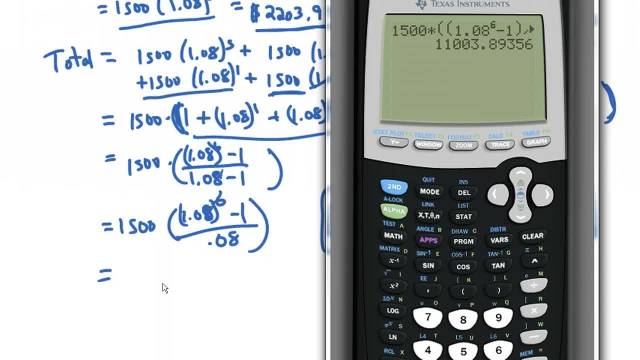 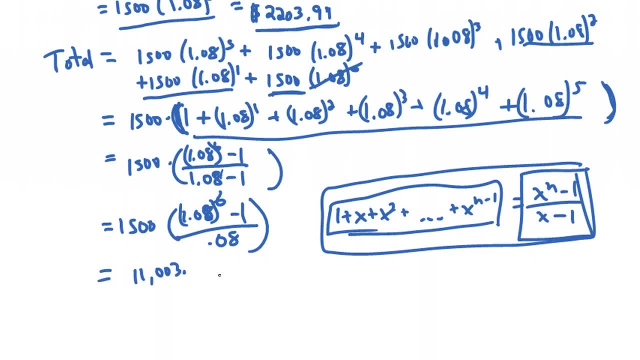 thousand, so we have a little over eleven thousand eleven thousand and three dollars and eighty nine cents, so let's write that in here: eleven thousand three dollars- and i already forget it- and 89 cents. okay, so that's the future value of this annuity, okay. the key part, though, was was figuring out. 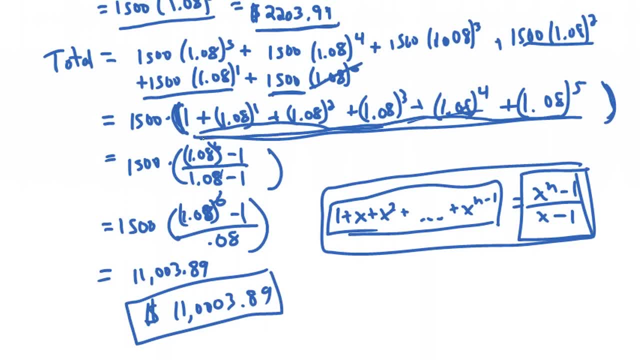 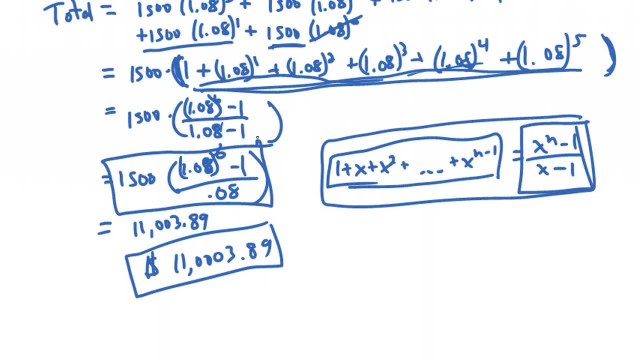 that this: when we added up all these terms here, we could use the formula from the previous video. now, one thing i want to point out is: let's look at this right here, in fact, let me, let me put it in in red right here. let's look at this and let's talk about the formula for the future. 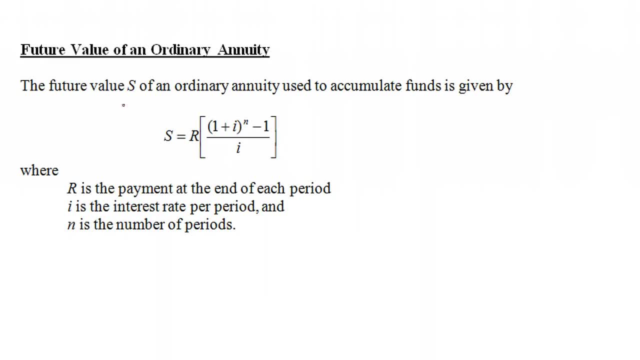 value of an annuity. this says the future value s. now. previously we've been using a- the future value okay, but we're going to use s when we're talking about annuities. the future value of s of an ordinary annuity used to accumulate funds is given by this: s equals r. 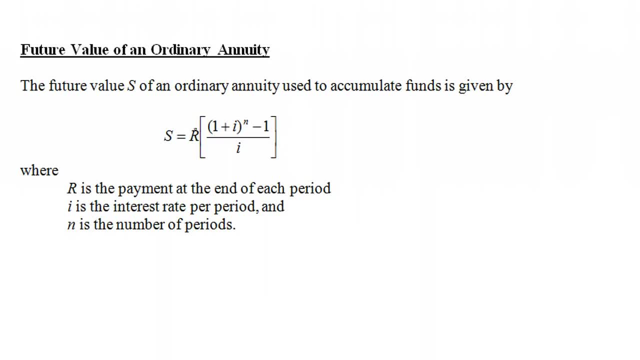 okay, where r is the payment at the end of each period. in our case, the r was fifteen hundred dollars, the i is the interest rate per period and n is the number of periods. well notice, is this essentially the same thing as what we had up above, remember, didn't we have that the future? 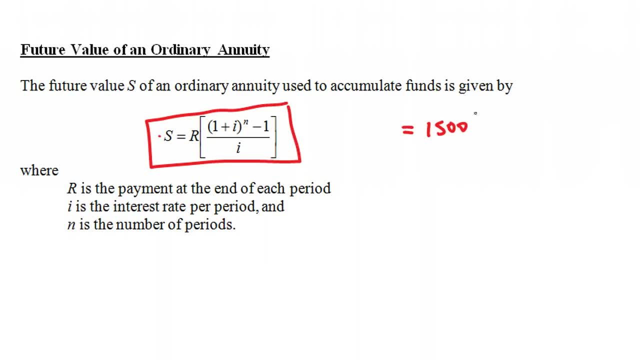 value was equal to fifteen hundred. okay, the r was fifteen hundred times. now i was using. there's no difference between brackets and parentheses. they're essentially the same thing, but one didn't. i have 1.08. that was 1 plus the i to the sixth power, right, so that's one plus i to. 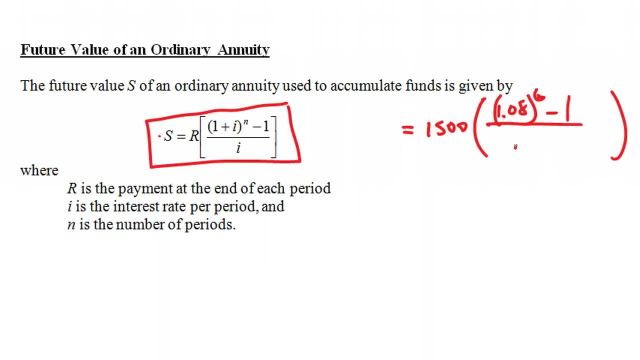 the six and we had a minus one. and what did we have in the denominator? we had 0.08. okay, so that was the i. so you can see this formula. this, this right hand side of the formula, chorus, corresponds to what we did here. okay, but really, where this formula ultimately comes from, was that?